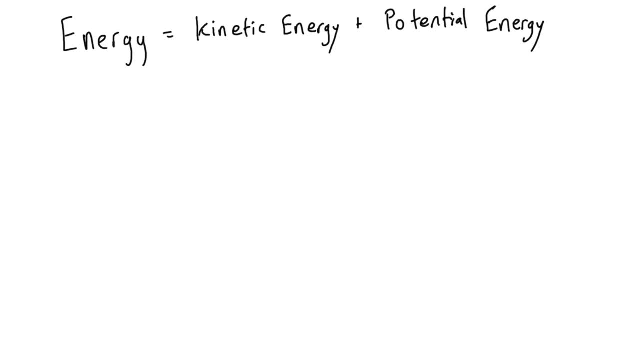 a moving force doing work on an object. when we have a moving force, it does work on an object. the energy that's imparted to the object is equal to the work done by the force. so that's a really important point, and I just want to make sure that you really, we really do get. 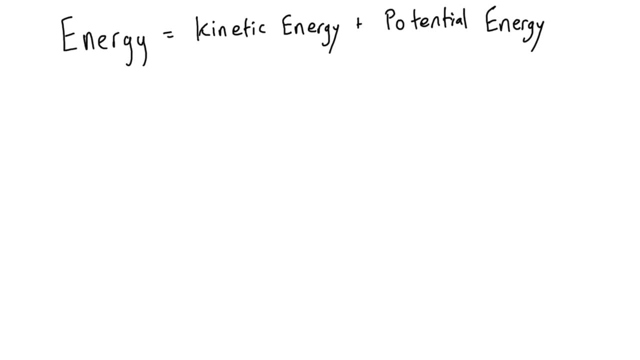 that. so when a moving force does work on an object, the energy imparted to the object is equal to the work done by the force. so what's happening in almost all of these problems is we're going to have like two states, like you know, point in time, one and point. 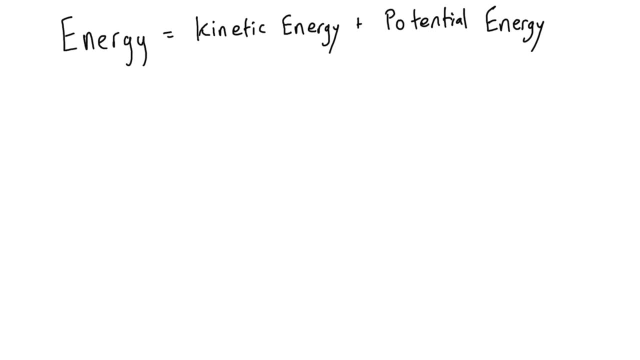 in time two. we're going to have energy- so the sum of kinetic energy and potential energy- at point one and we're going to do some work on the object, and then we're going to have point two in time, where we're going to have a different amount of energy and the difference is going to be the. 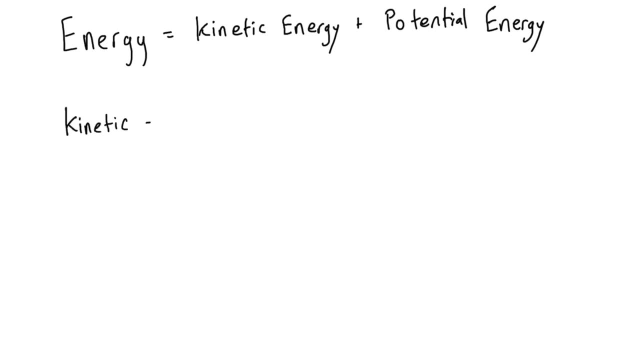 work that was done. so the expression for kinetic energy is just capital T- that's how we refer to kinetic energy- is equal to one half mv squared. I'm assuming most people have seen this in high school- it wouldn't be new, but it's definitely worth committing to memory as you're studying Dynamics. 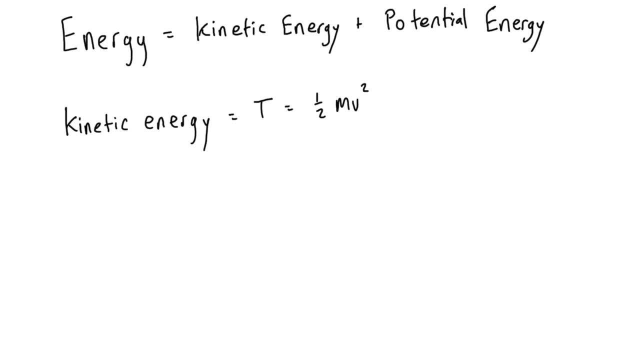 or at least this section of Dynamics. but yeah, so kinetic energy is completely related to the motion of an object and specifically it's related to the speed of the object. we have that term in there for velocity- super important that it's there. while we're here, let's talk about units. so m is mass. 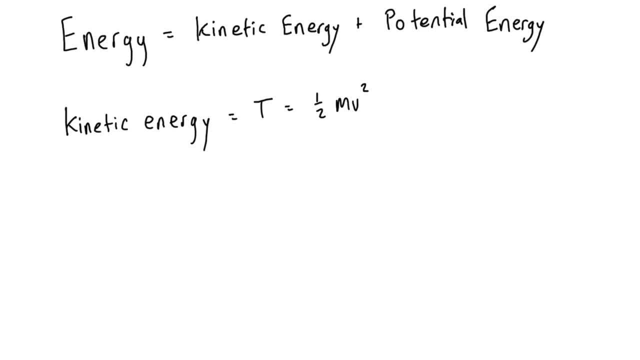 in kilograms. actually I'll write it on the side. so m is mass in kilograms and v is velocity in meters per second, and that's all squared right. so that means we have kilogram meters squared per second squared, which is the same thing as kilogram meter per second squared. 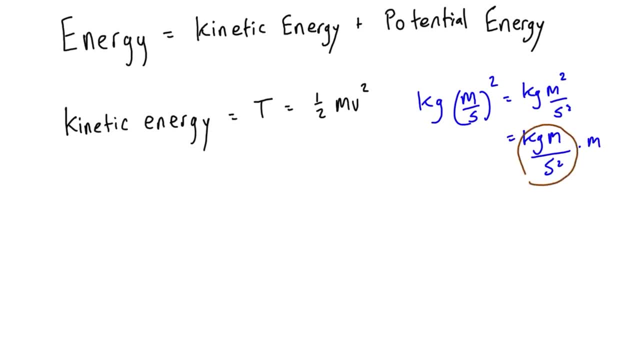 times meters and this first part, this first part, right there is Newtons, so that's equal to Newton meters, which is equal to Joules. now, when we're talking about potential energy, we denote that with a capital V, and we actually are in these mechanical problems, are going to split it into potential energy, gravitational potential energy, so vg and also. 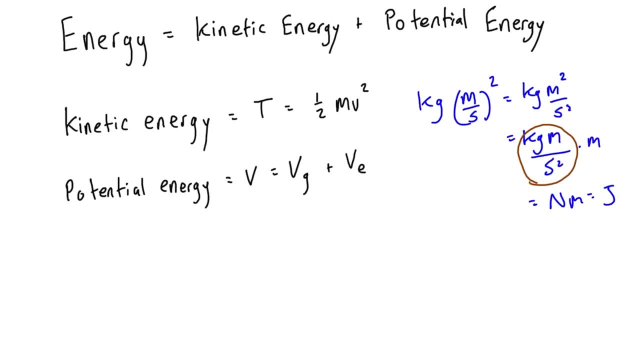 elastic potential energy, ve, this referring to Springs, the elastic potential energy of Springs. so this whole expression, v is equal to vg plus ve is referred to as the potential function and ultimately, potential energy in general is for conservative forces and it's related entirely to the initial and final position relative to a. 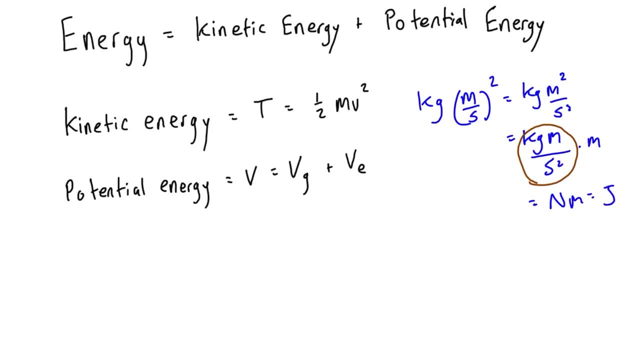 reference that we choose. it's going to be a different reference for gravitational potential energy and spring potential energy or elastic potential energy, and you'll see that in one second. so let's write the expression, I guess, for gravitational potential energy first. so we've got vg and this is just equal to m g h. I think most people probably have seen this again. 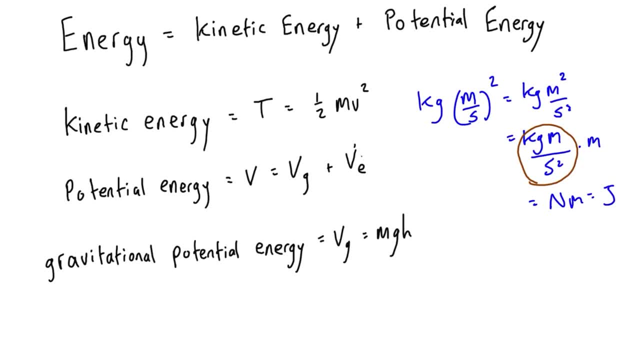 in high school level course, um. m is mass in kilograms, g is acceleration due gravity and H is height in meters. you might see this written sometimes maybe, as wy w just referring to mass times, gravity, so mg and y just being another way to write H for height. and if you do want, 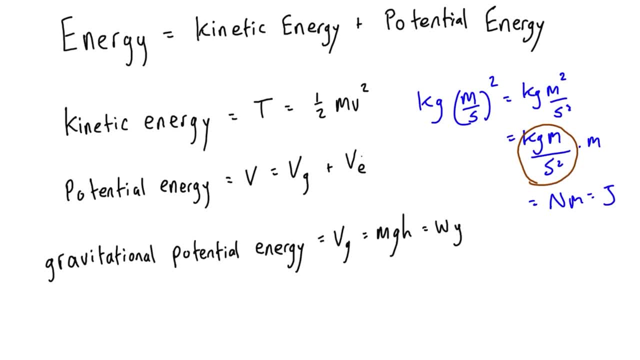 to talk about units here. just to confirm that this isn't units of Joules. again we have kilograms- Acceleration due to gravity is meters per second squared and height is in meters. And again we have this kilogram meters per second squared, which is equal to newtons. 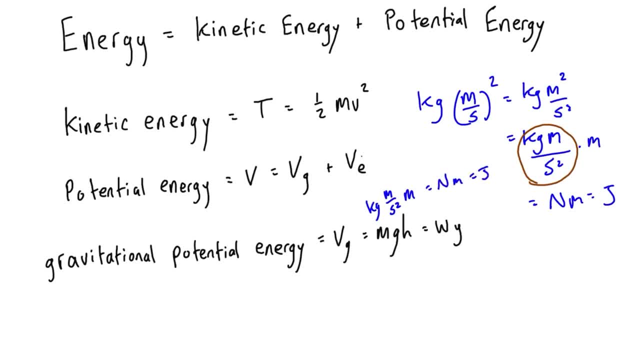 and then times that meters, which is equal to joules. Or if you've already converted mg to weight, then weight is in units of newtons and y is meters, so again joules. All right, and then just the expression for elastic potential energy is v, e, which is equal to positive one half k, x, squared. 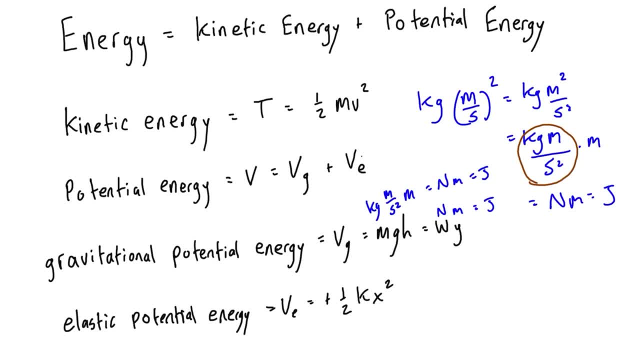 Now, it's always positive because whether we're stretching or compressing a spring, the spring force will always be directed towards the unstretched position. It always wants to return to that position. It's always going to give you a positive value, And then, for the rest, we have.